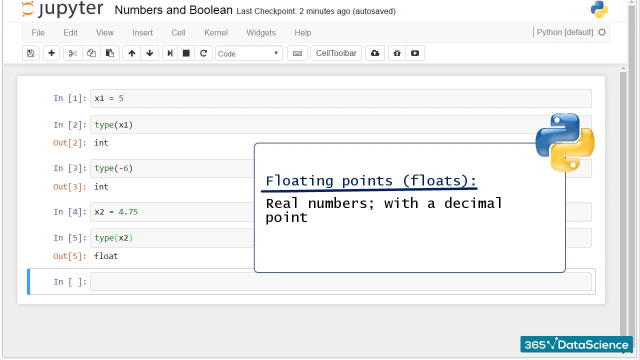 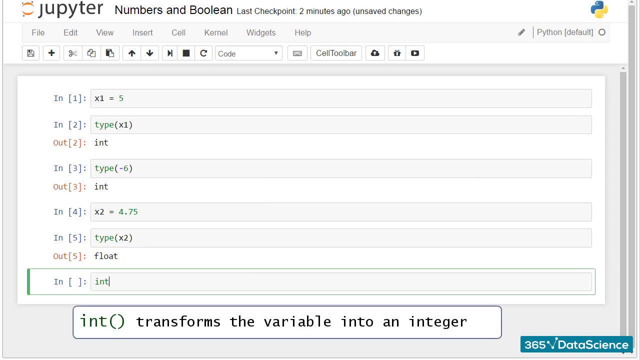 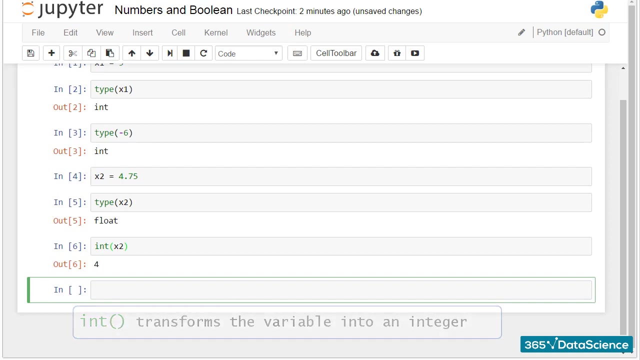 are real numbers, Hence they have a decimal point. 4.75 is such a number. Therefore Python reads it as a float. Let's look at two other built-in functions. Entãoelessverfort, его iPhone somado Beautiful. 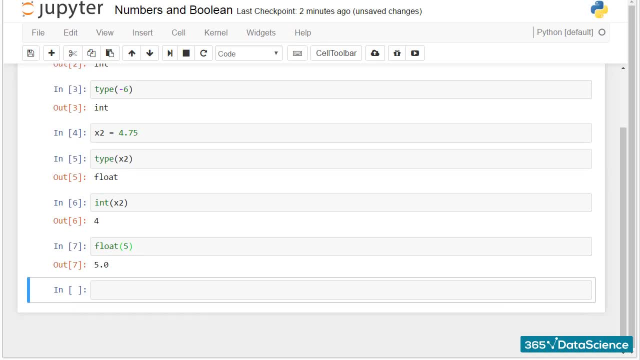 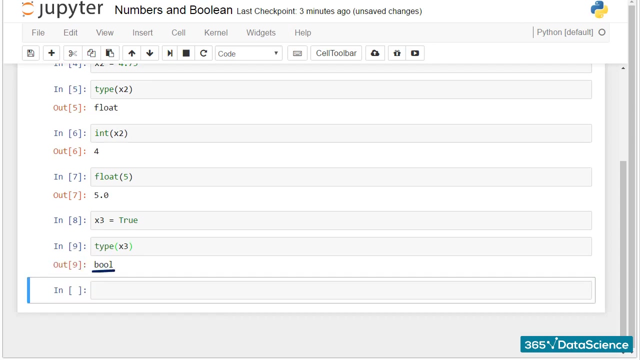 intestinal Integer, Integer, Integer, Integer, Integer, corresponding to the machine's logic of understanding ones and zeros: on or off, right or wrong, true or false. Let's provide an example with a new variable, x3, which is equal to true, Right. The output of the type function is bool, which simply means x3 is a boolean. 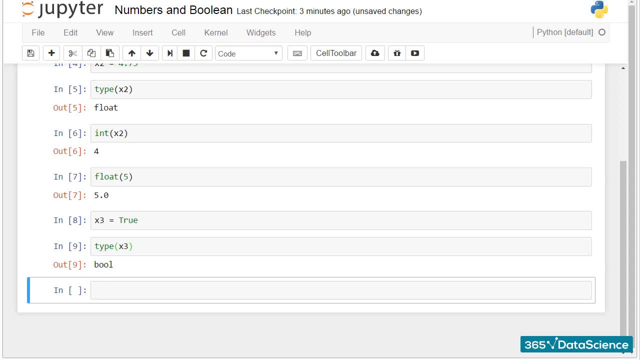 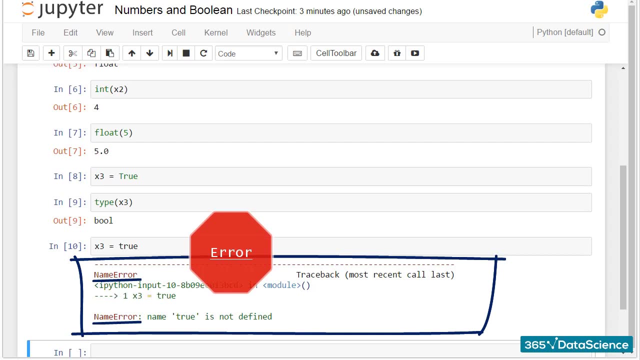 An important detail you should remember is you have to type true or false with capital letters, Otherwise Python won't recognize your variable as a boolean and will display an error message. So, to wrap it up, the two boolean values a variable can have are true or false, and they must be written with capital letters. 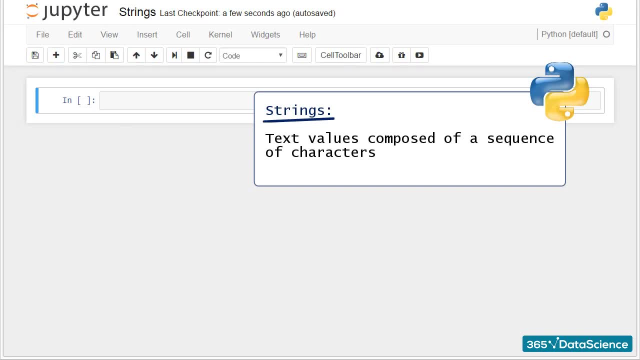 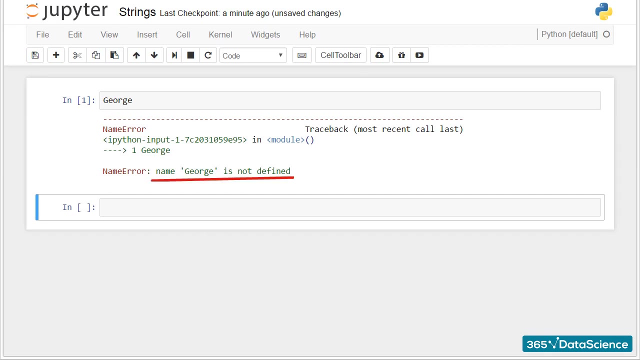 Strings are text values composed of a sequence of characters. Let's see how we can create a string in practice. If we ask the machine to display the name George, this way we'll obtain an error message. Why? Because Python assumes George is the name of a variable to which we have assigned no value. 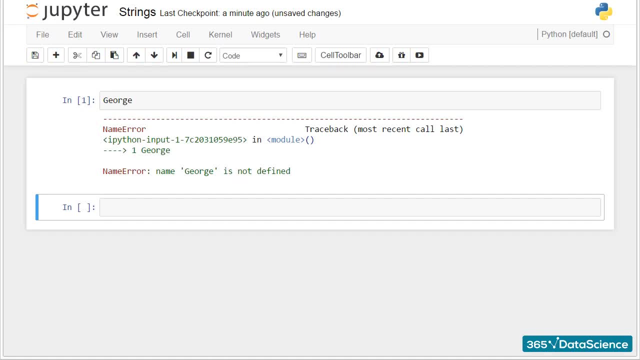 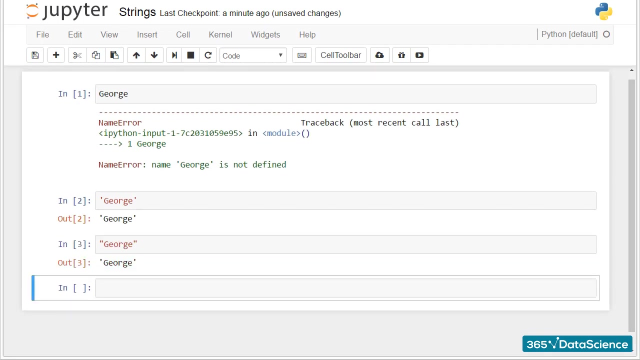 Here's the magic trick that will correct this mistake. Let's type single quotation marks around the name George first, And now let's type double quotation marks around it. You see, the output values of these two inputs are the same. This is how Python displays text results if you don't use the print command. 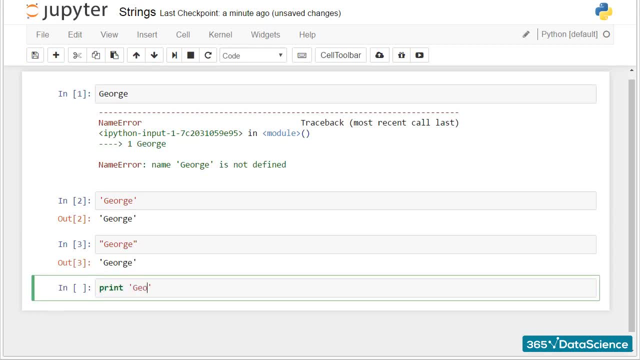 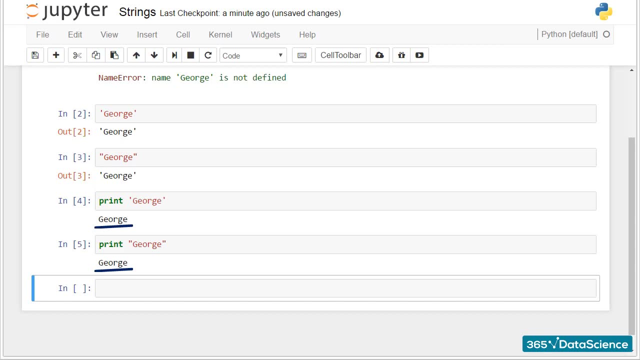 Should you use print, the output will be shown with no quotes. You'll be able to see plain text. If we assign this value to a new variable, let's say x4,, we can obtain its output as we did with the integers and floats. 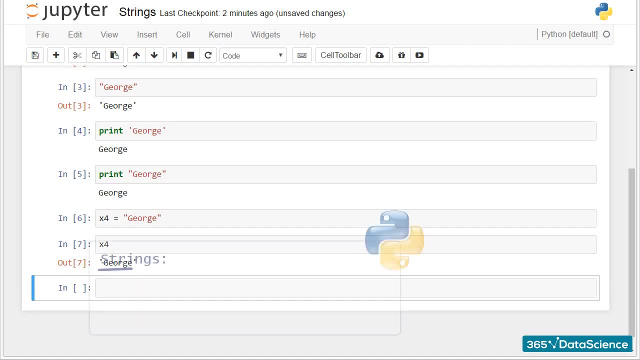 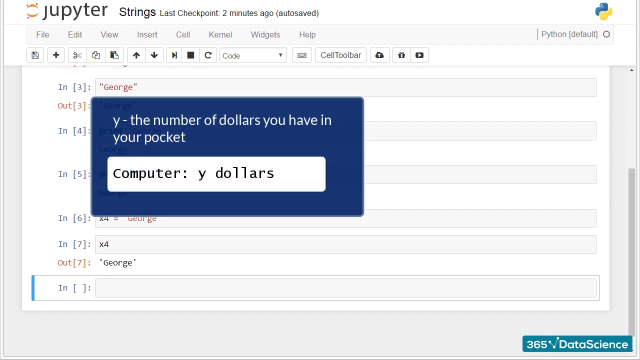 Alright, so that's it. If the values you'd like to assign are not numerical, the quotes can come into play, Assume the variable y is supposed to represent the number of dollars you have in your pocket. In addition, you would like to ask the machine to print out a statement that says y dollars. 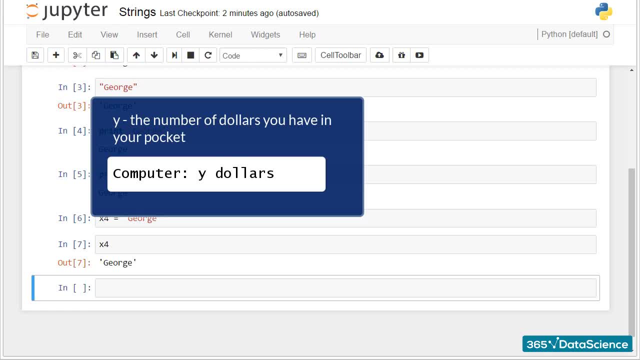 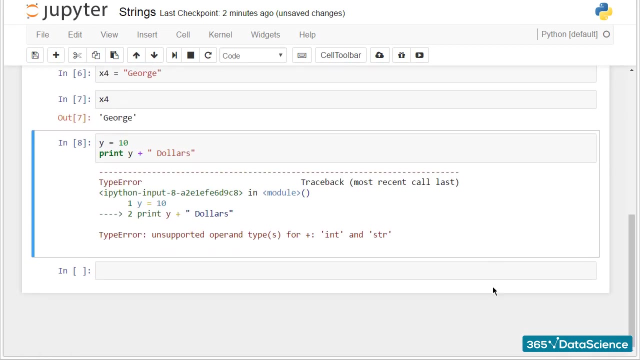 where y is a number, The proper way to combine the value of y and the string dollars is to use a plus sign, as shown here. Let's execute this cell to check if we are missing something. Apparently, we did not respect the rules of coding in Python. 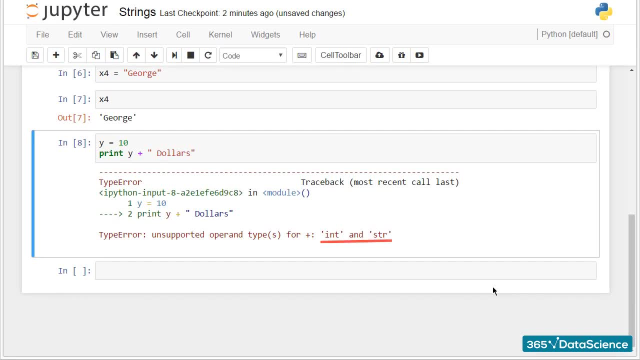 We cannot put different types of variables in the same expression. y is an integer and dollars is a string. We can convert y into a string. String is the built-in function we need, Analogically to integers and floats. string will convert our number into text. 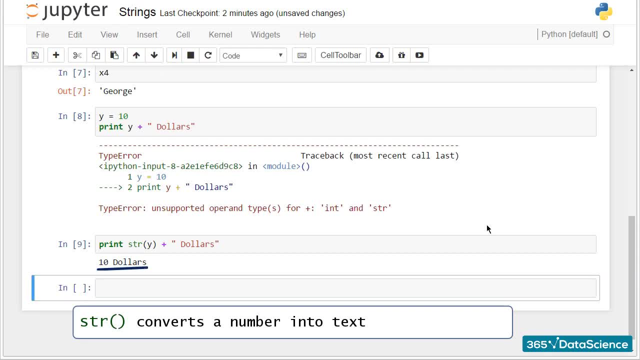 and that will unlock our result. To summarize what we said so far, Python can automatically guess the type of data you are entering. It is within its capabilities to know for sure whether you have assigned an integer, a float, a boolean or a string. 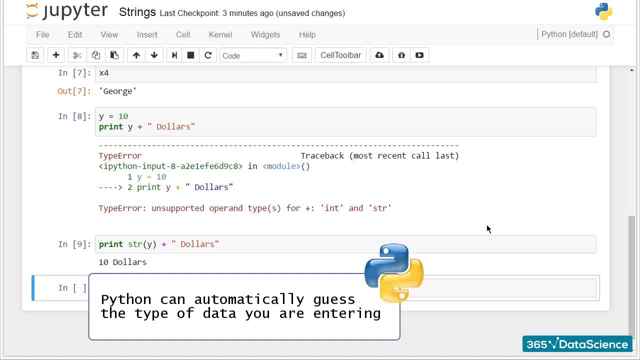 You need not declare the types of variables explicitly, as you must do in some other programming languages. Python always knows the type of variable. What will happen if you type something like I'm fine, You'll need the apostrophe in the English syntax. 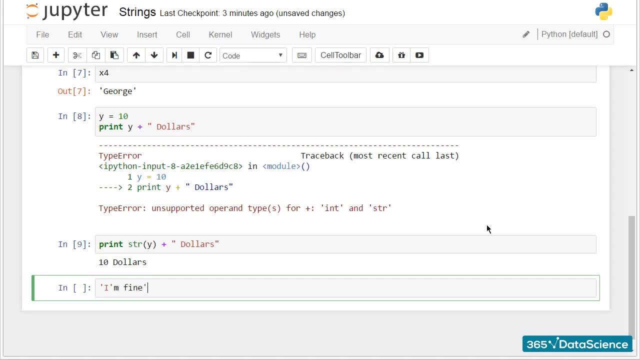 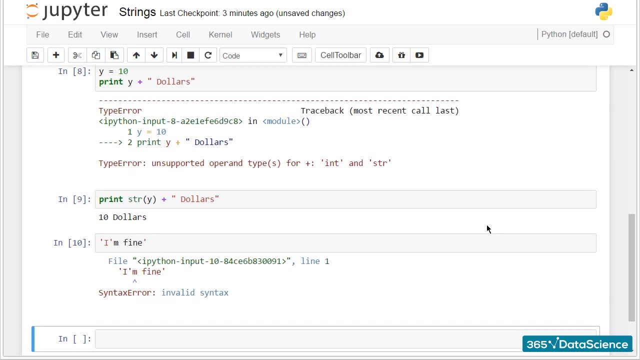 not for the Pythonic one. Observe: if you execute the command like this, you will make a mistake. To avoid that in such situations, you can distinguish between the two symbols, Put the text within double quotes and leave the apostrophe. 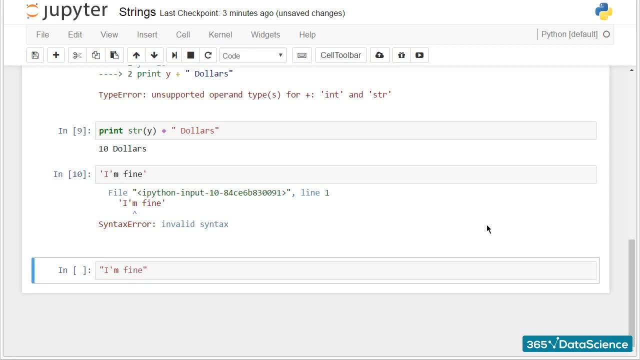 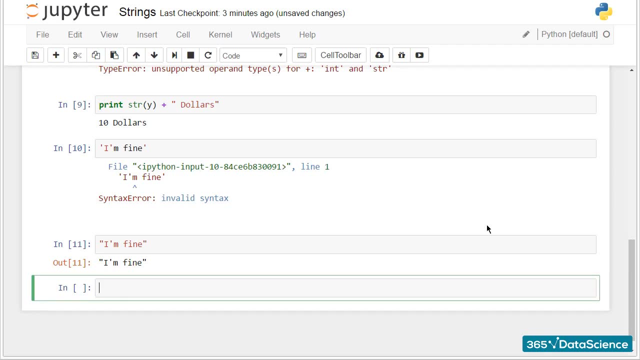 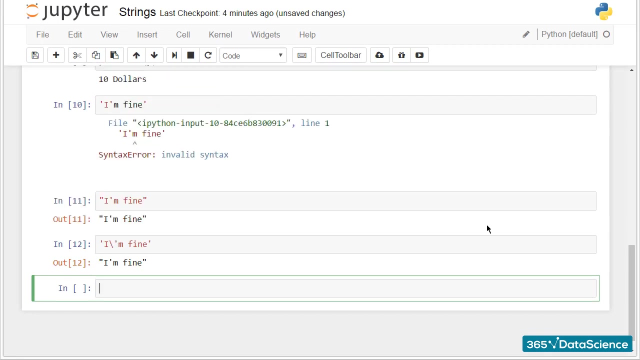 which technically coincides with the single quote between i and m. Now you are fine. An alternative way to do that would be to leave the quotes on the side and place a backslash before the apostrophe within the phrase, and we'll still obtain the same correct result. 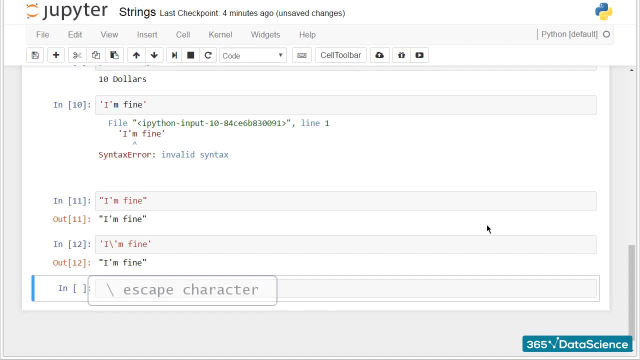 This backslash is called an escape character, as it changes the interpretation of characters immediately after it. And what if we wanted to state press enter, where we put enter within inverted commas? Same logic: the outer symbols must differ from the inner ones.